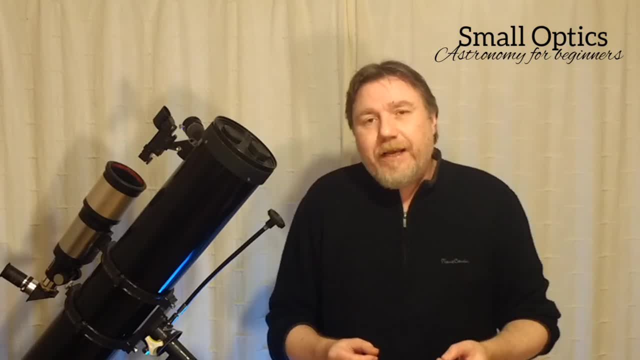 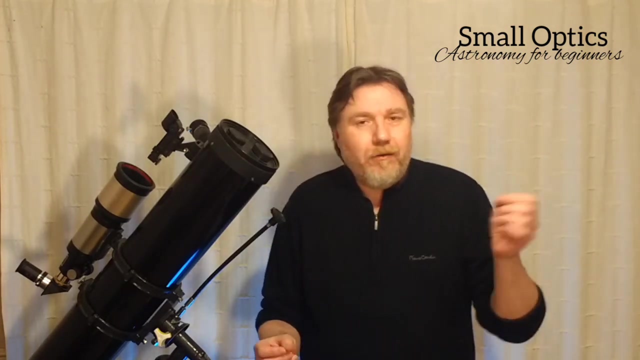 And get yourself organised. Get all the eyepieces that you're going to be needing together. Maybe that flashlight. Now, one thing you don't want to be doing is keep nipping into the house for you know that eyepiece that you may have lost, or that warm cup of tea, or something. 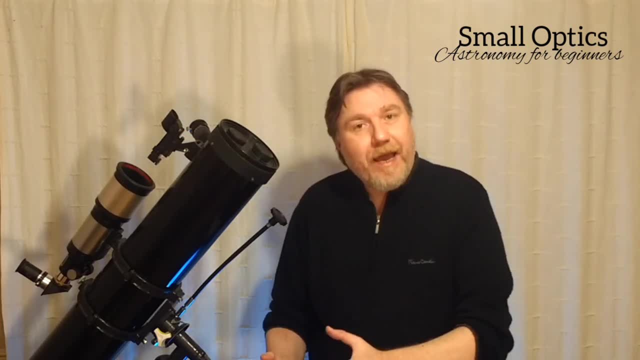 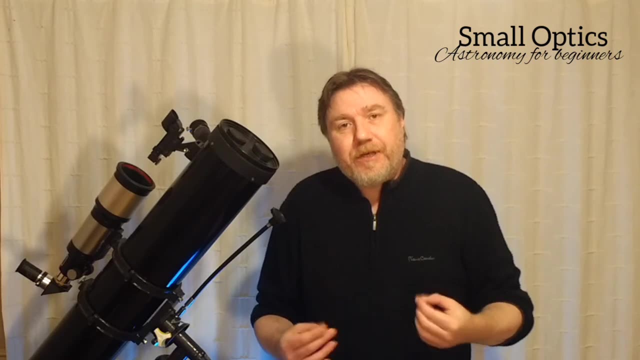 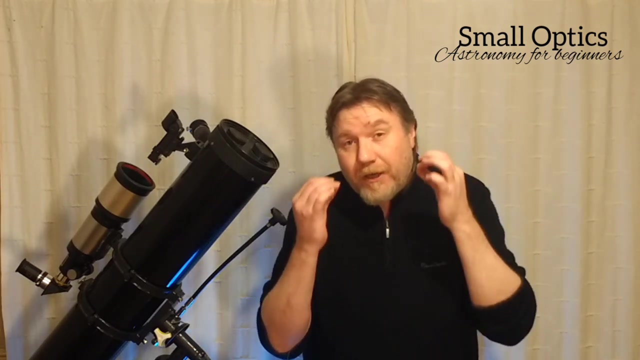 Have a flask, Take it outside with you. Have everything prepared and ready to go, Because what you need is to get what they call dark adapted eyes okay, And this can take up to 20 to 40 minutes to get your eyes properly dark adapted. 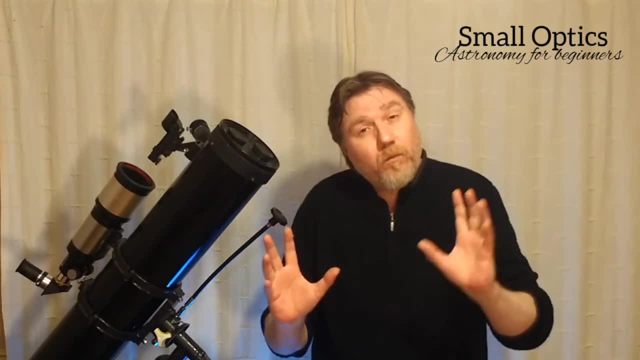 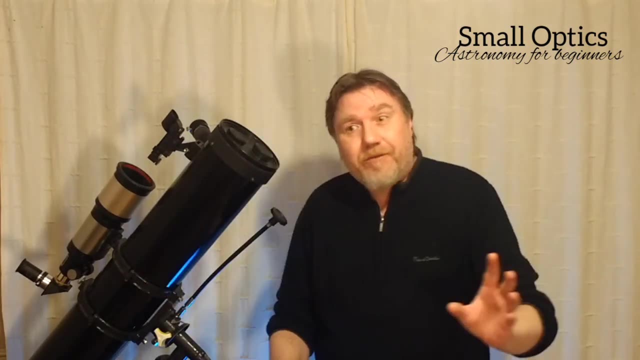 So you can see a lot, A lot better. You'll see when you first go out. when you look at the sky, it doesn't seem quite you know as many stars as after maybe being out there half an hour or so. 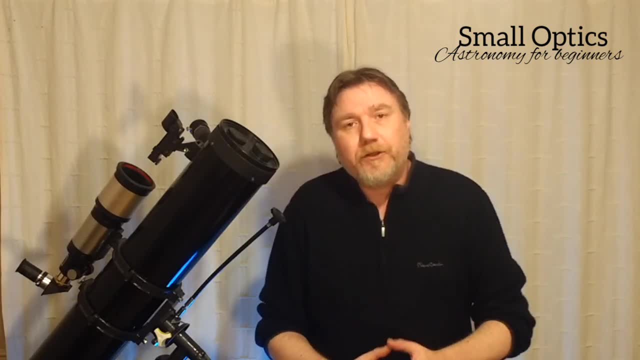 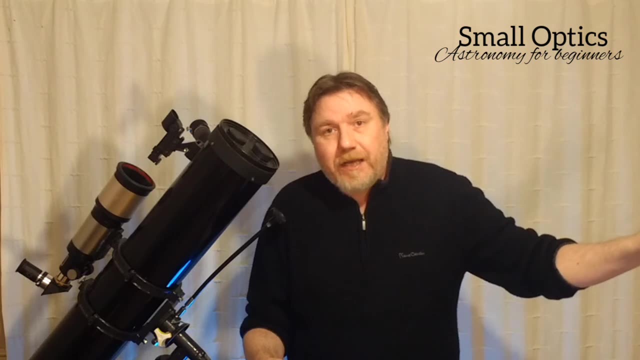 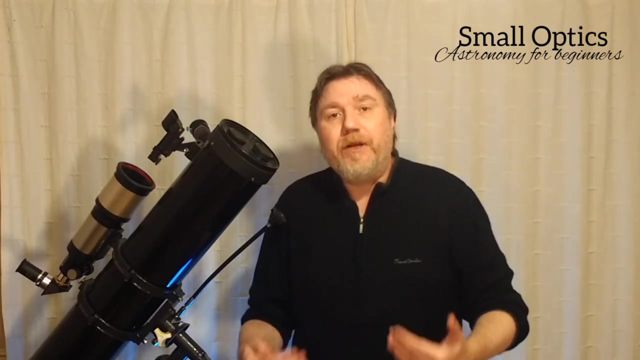 And then all of a sudden, the sky seems to be full of stars, And that is your night vision, if you like, And nipping inside the house under artificial light will just zap that away in an instant, okay, And it's going to take another 20 to 30 minutes for your eyes. 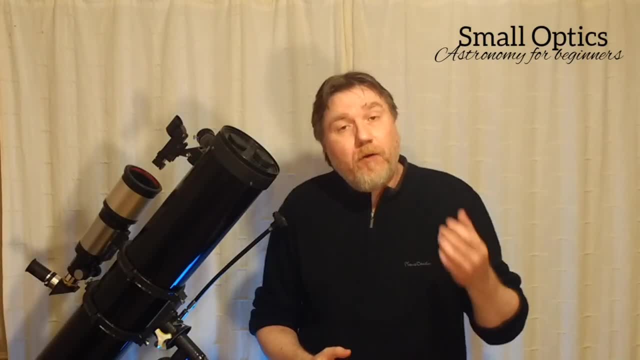 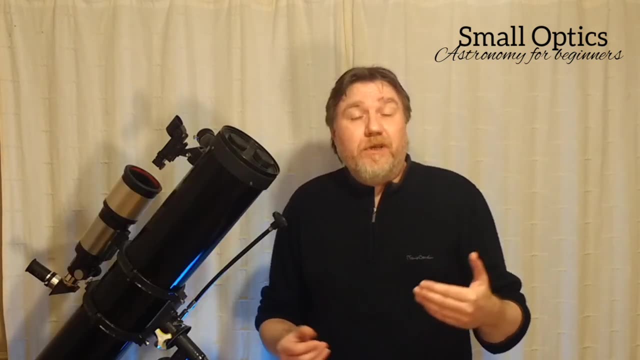 To get accustomed to the dark. You could also arm yourself with a red light torch. These are easily found on the internet. You could even make these out of ordinary torches and just put a couple of layers of electrical tape- red electrical tape- on. 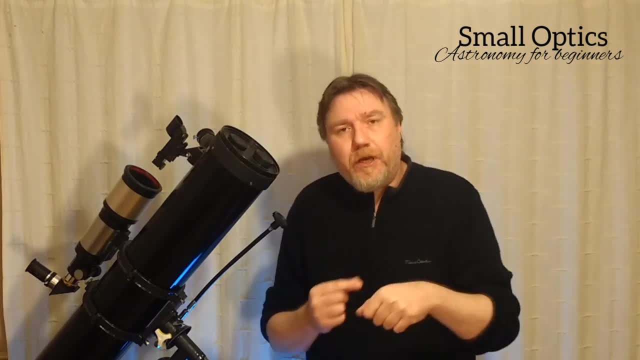 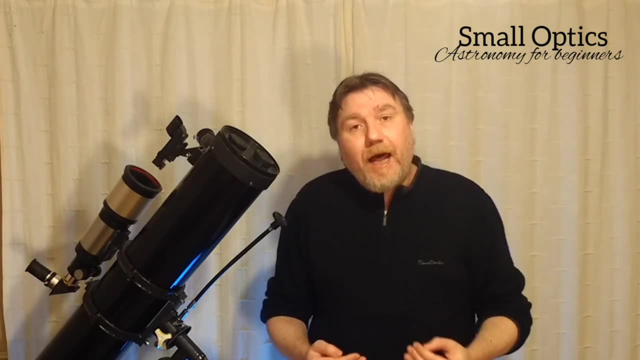 Some people actually like to use brown tape, But I always use red electrical tape on ordinary torches And that seems to get that light factor down, Because red light is kinder on our eyes than the harsh white. Okay, tip number two: 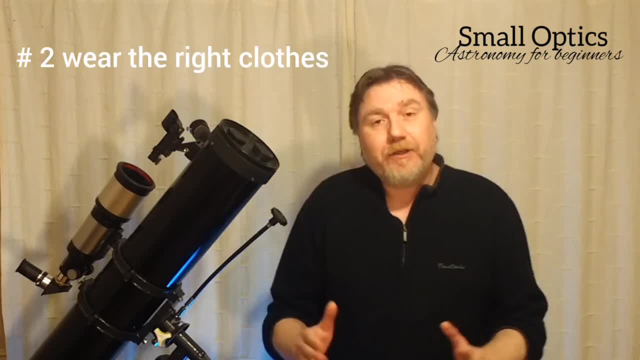 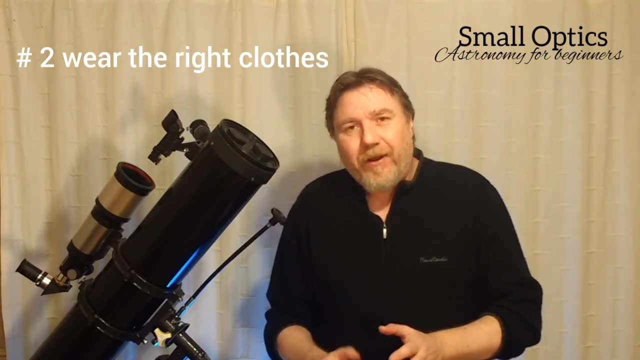 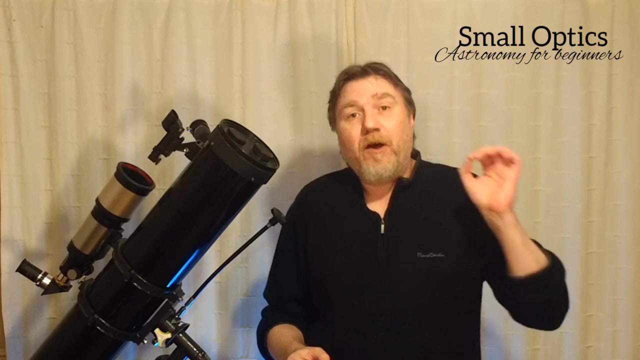 Dress correctly. okay, It's so important. A lot of newbies to the hobby. that's one thing. They underestimate the weather. okay, Always look at the conditions. If it's cold out there, if it feels cold when you first step outside, it's going to feel freezing after about 10 or 15 minutes. 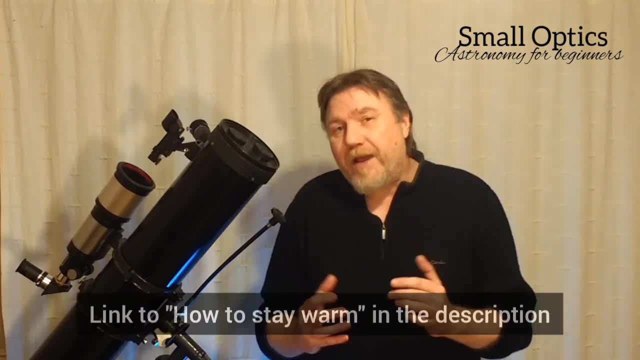 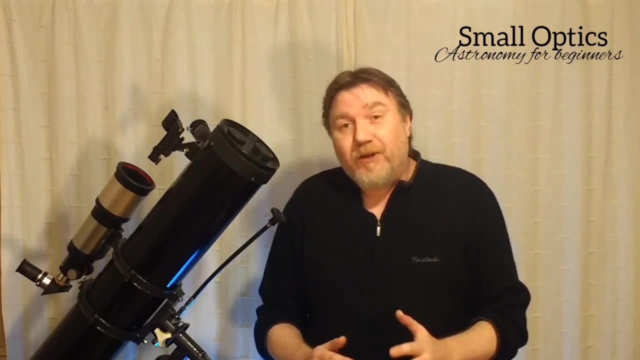 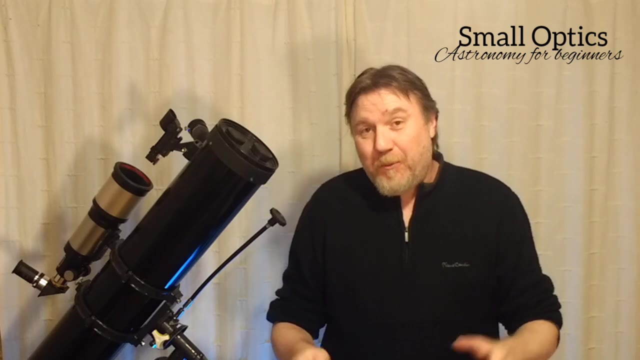 So I have a full video on the correct way of staying out there all night. But it's really important And something you don't want to overlook is putting the right gear on for those cold nights. Number three: Never use your telescope indoors, okay. 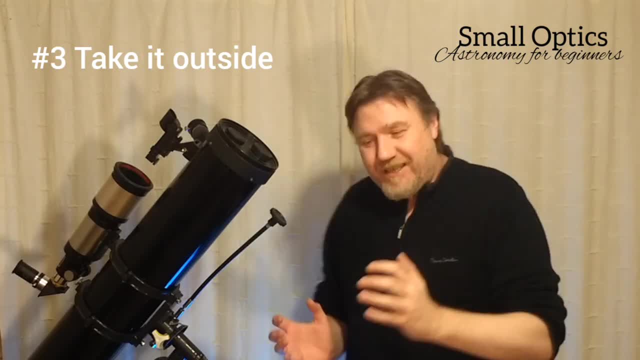 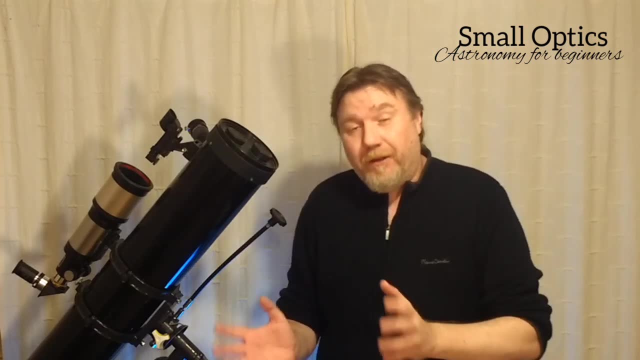 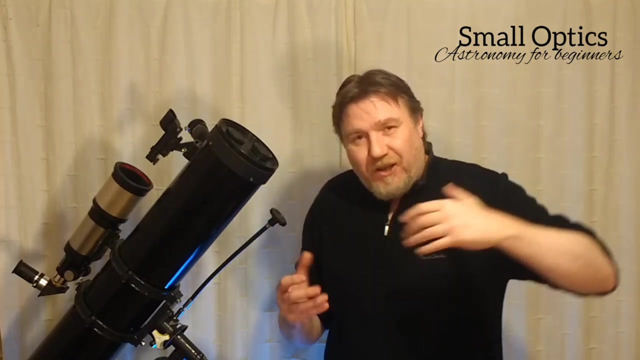 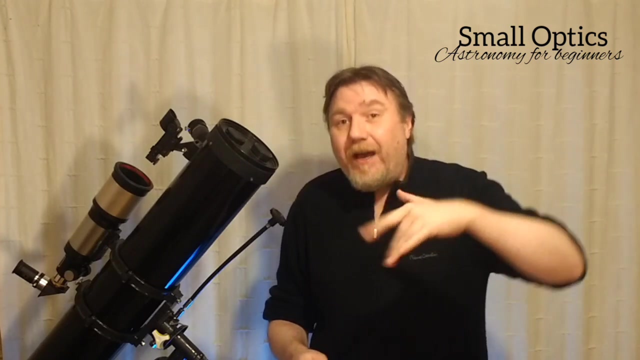 Now, what I mean by that is: don't sit inside in the nice warm, open the window, okay, And point your telescope through the window, Especially for astronomical viewing- Well, this is mainly for astronomical viewing. Well, what will happen Is, as all the warm air is flowing out of your nice warm house, it's going to be hitting the cold air and you're going to get that wobble effect. okay, 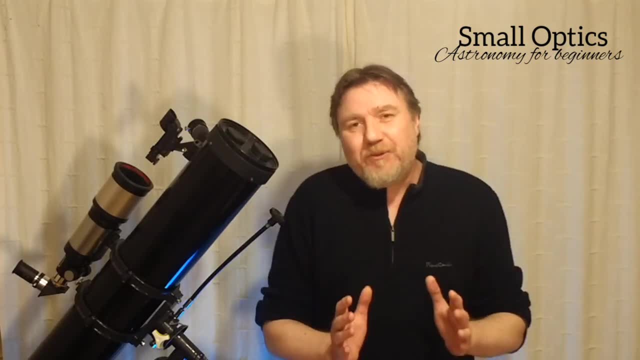 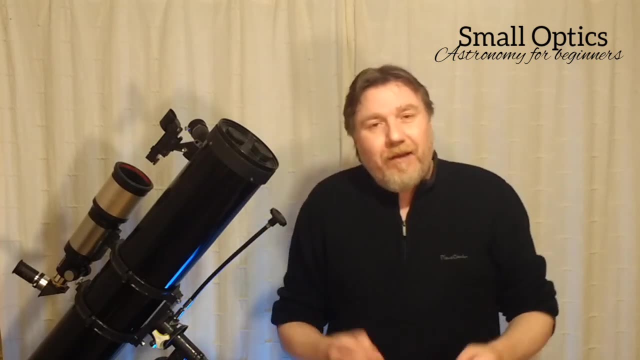 And everything, you'll just not get no focus. What you've got to remember is telescopes are designed to be used outside, okay, And that includes looking through windows as well. I mean, I know some people that you know say I just can't get focus. 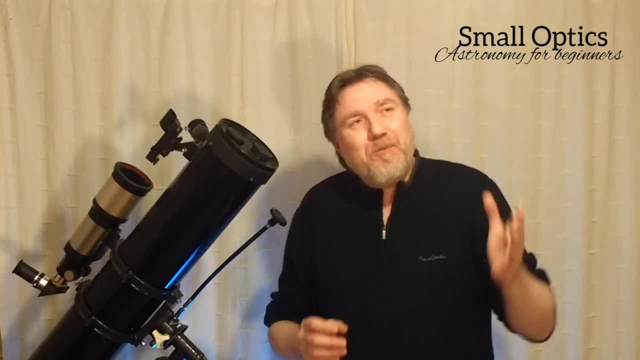 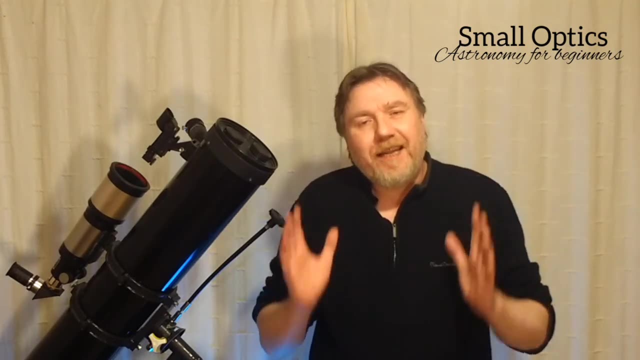 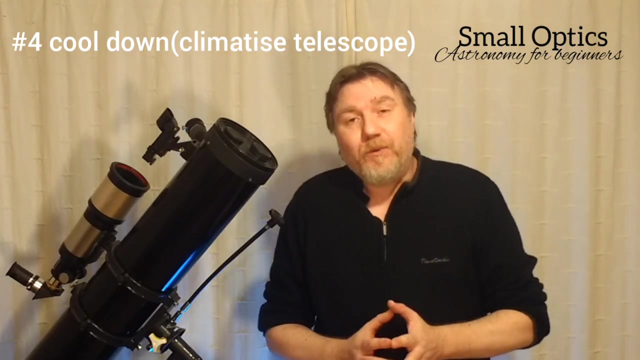 And there was actually. I had the telescope set So under the skylight in the room I see just looking through double glazing. Number four: Always allow your telescope enough time to cool down. Okay, Now, this is another thing overlooked by people new to the hobby. 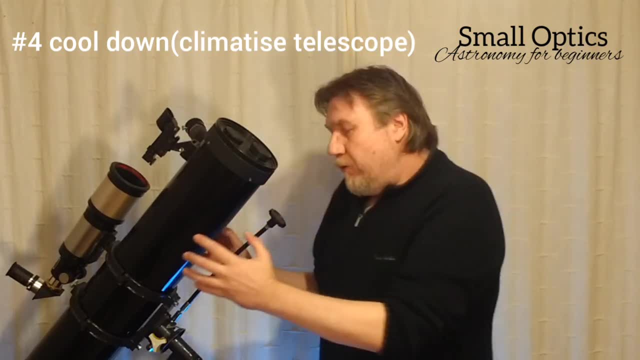 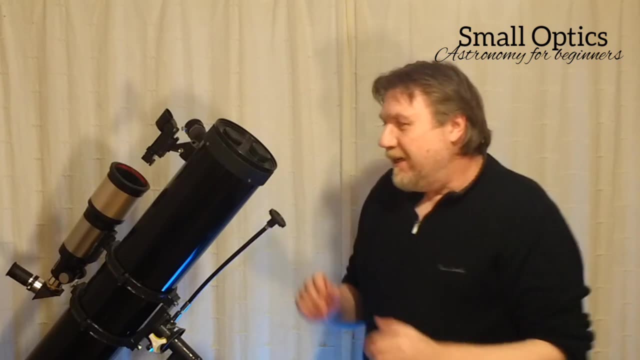 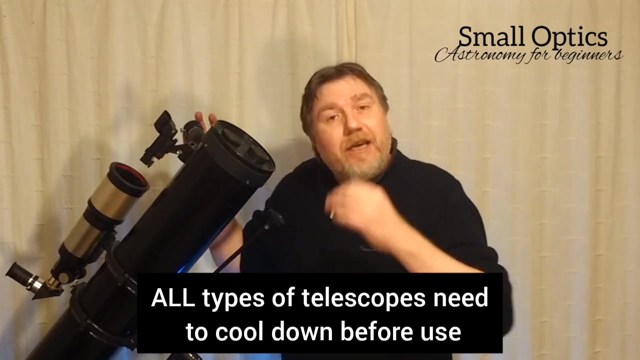 Um, now inside the tube. Okay, If you take outside your telescope, uh, in our, from a nice again, from a warming inside to the cold outside, the warm air that's trapped inside the tube, Well, actually It will interfere because we're using quite high magnifications, will actually interfere with the uh, you'll get the thermal effect. 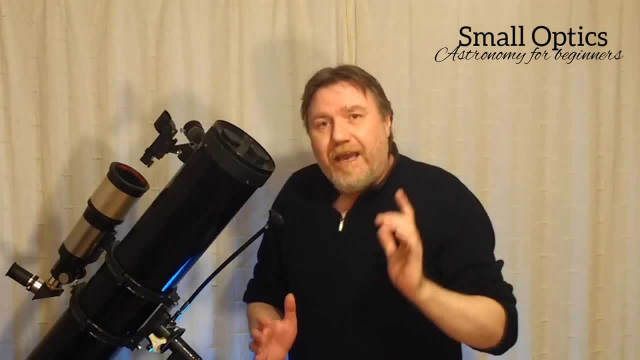 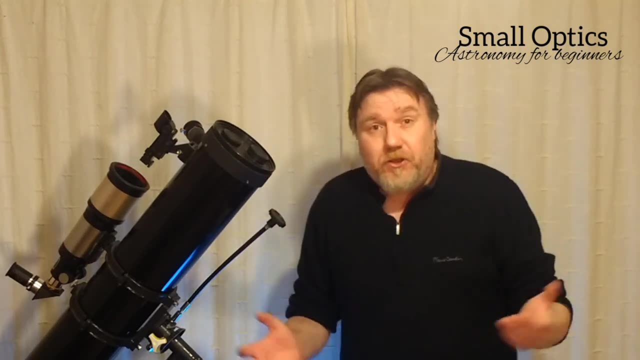 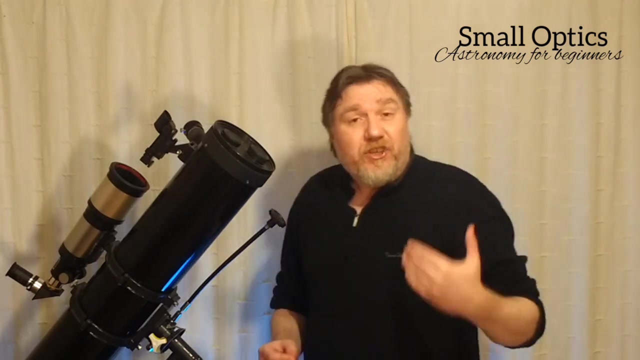 Okay, Uh, and it'll be again a wobbly image. So it's really important to take your telescope out a good uh 20 minutes, uh to two to an hour really, to just let your telescope climatize to the cold uh outside or or to the same temperature, um, as what the uh temperature is outside. 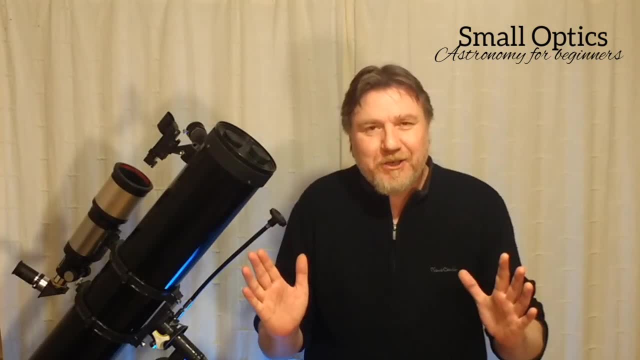 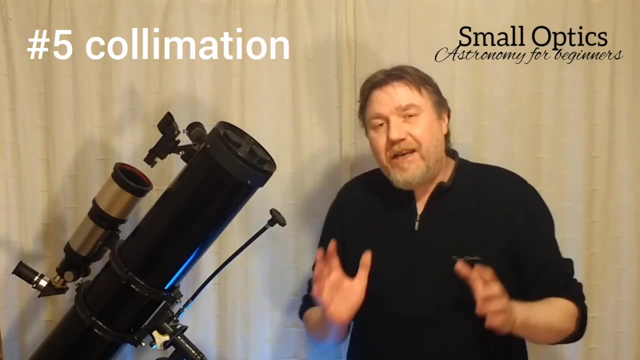 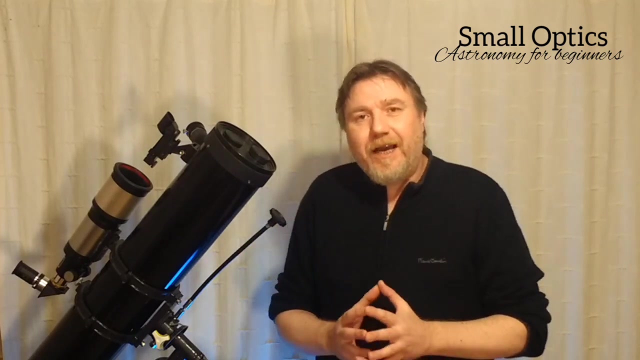 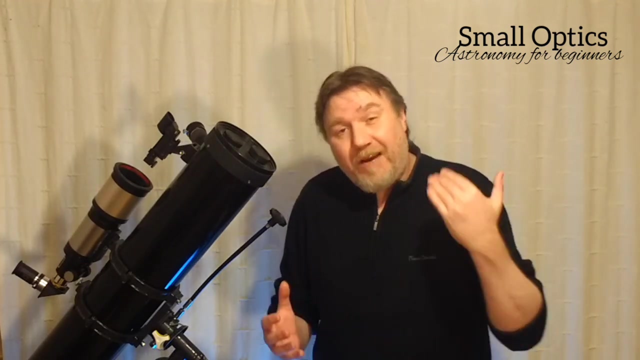 Okay, Number five, Let's get it out of the way. Collimation: Okay, Now, this is purely for reflector users. You got to make sure that your telescope is in good collimation. Um, now, don't think that. uh, you know, if you are a new telescope owner and your telescope hasn't been collimated even after, maybe, uh, a month or two after first buying it, then you better start thinking um again. 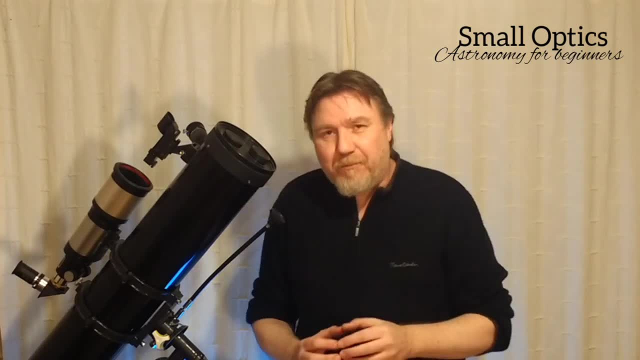 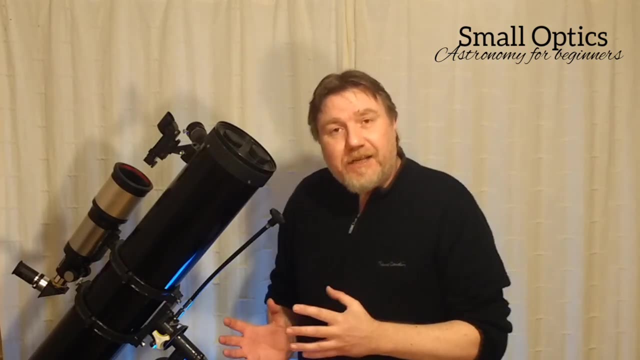 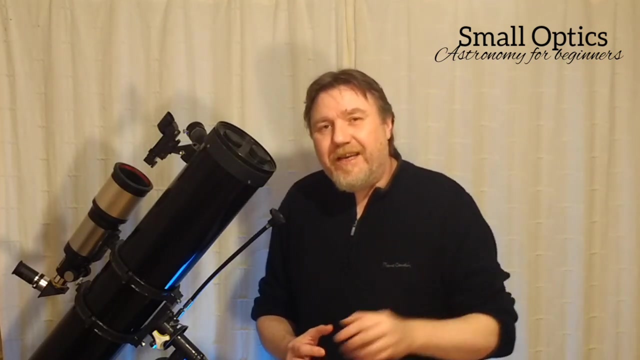 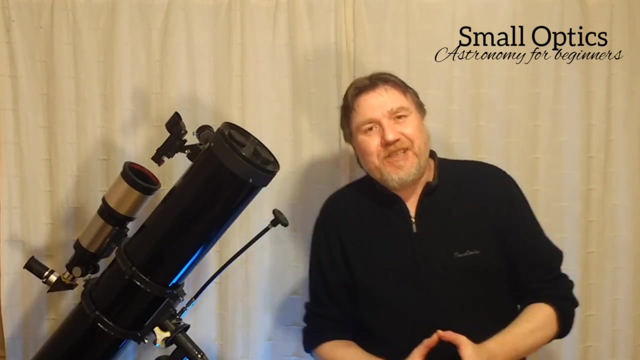 Okay, And uh, looking into collimating it pretty quick. Now I have got a video on um how to collimate a telescope, a reflector telescope, and it's a no laser method, a really easy method. So again I'll leave a link to uh, that one in uh in the description below, number six get to learn the sky conditions. 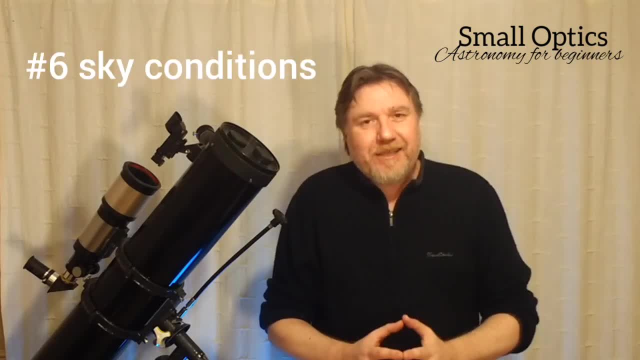 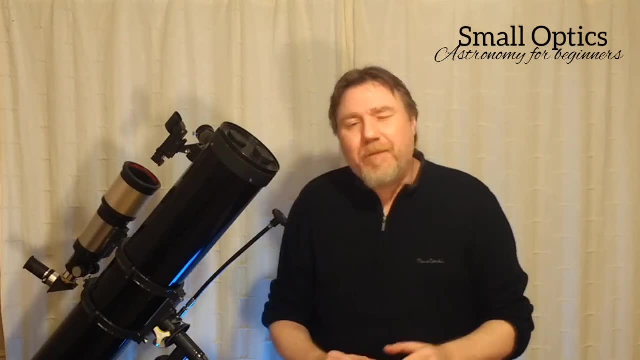 Okay, Now it's all right Looking at the weather forecast and saying, oh, it's going to be a nice clear night tonight, but sometimes You know it's that's still might not be the best time. And there's an easy test you can do. 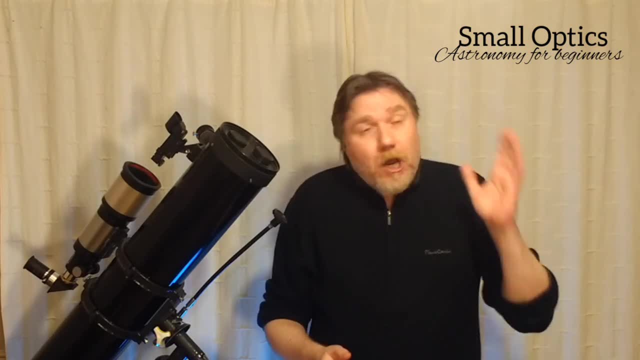 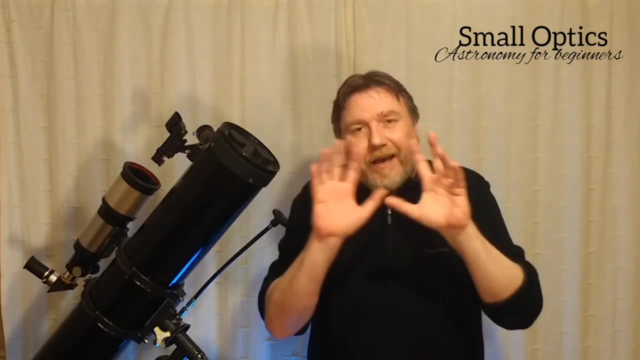 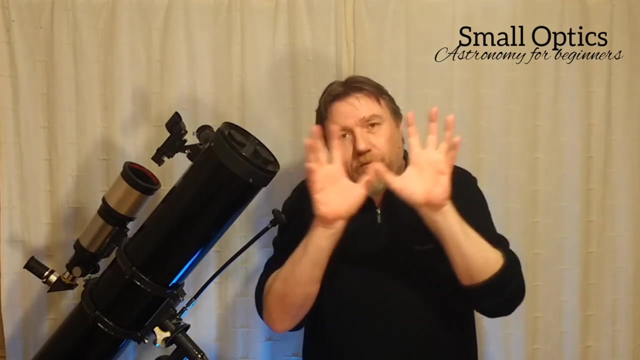 Um, and if you go outside on a nice clear night and look at the stars and see how they're twinkling, Okay, Now if they're quite vigorously going like that, it usually means that the atmosphere is quite unstable. What you're looking for is the stars to kind of move in a nice soft, undulating pattern. 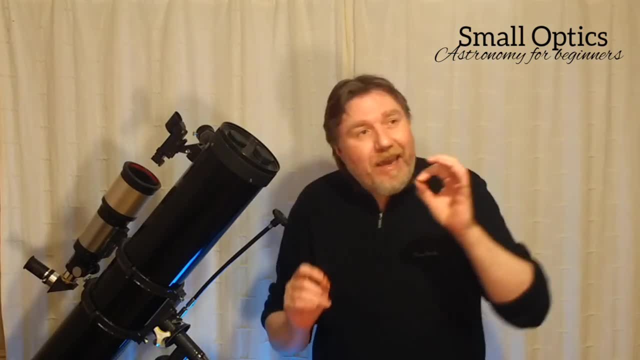 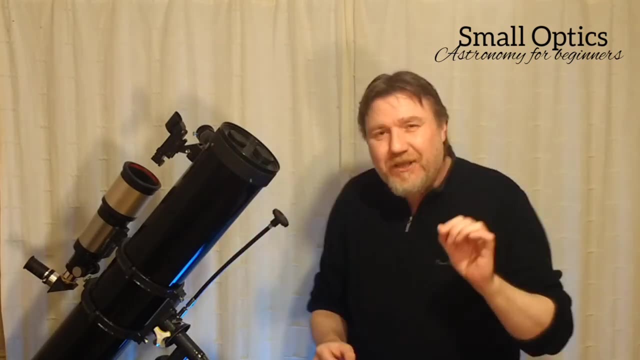 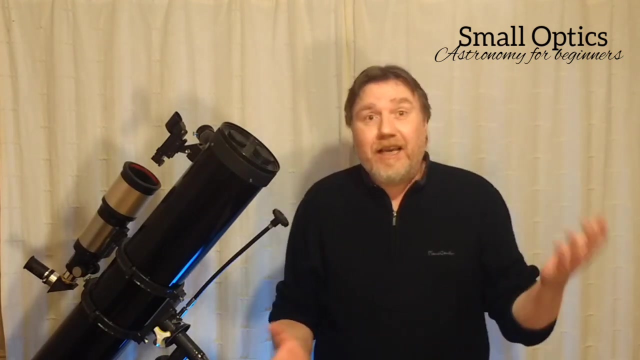 Do you know what I mean? And uh, also a nice if there's A little bit of mist in the air. Okay, Um, just just a fine bit of mist in the air. That's usually means that the atmosphere is really stable and it's perfect for viewing the planets and even the galaxies. 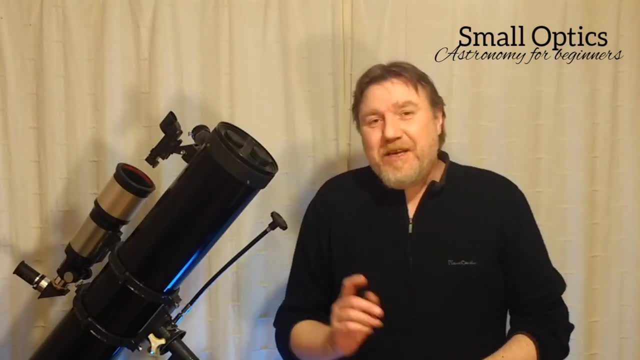 Well, astronomy, and okay, Tip number seven. Now this one. uh, maybe a bit of a surprise to some of you if you've never heard of this before. and that is when you get up to the eyepiece, keep both eyes open. 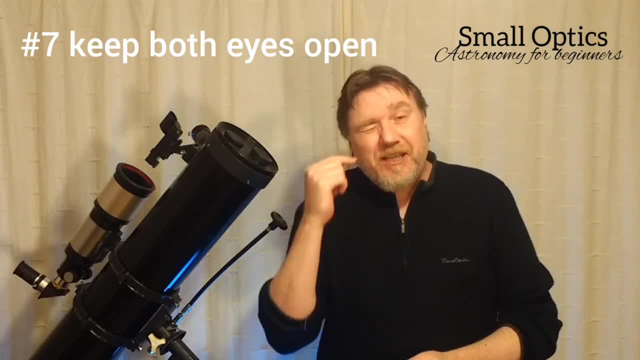 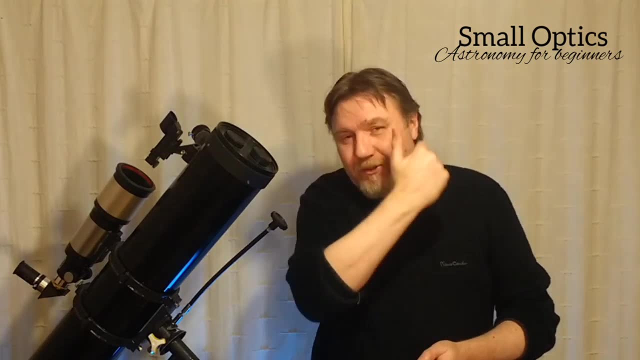 Okay, Because what happens is when you actually do this at the eyepiece and you're squinting and uh, looking through the eyepiece, that actually sends electrical impulses across, uh, to the other eye, actually makes the eye, brain, eyeball vibrate a little bit. 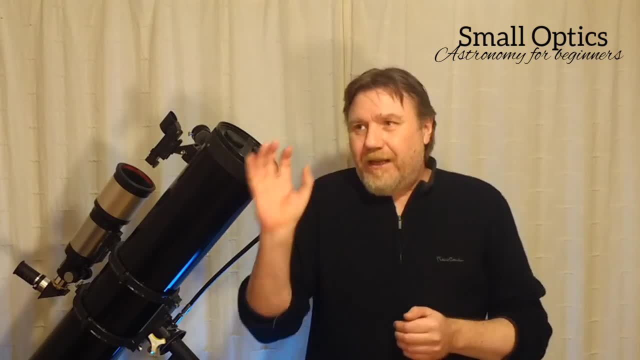 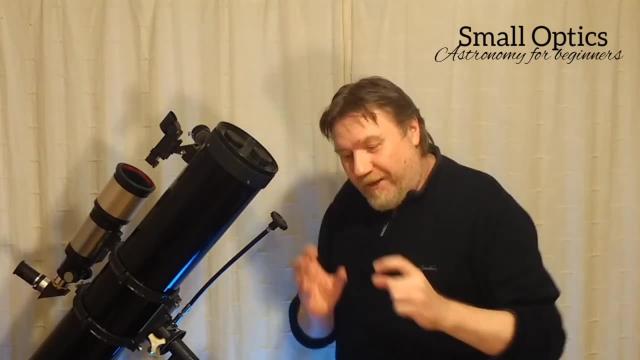 Um- and this is one of the reasons why you tend to think that you've got a better image in by no viewers- uh, which are a little bit like, um, binoculars that fit into the eyepiece of a, uh, of a telescope. Um- and this is one of the reasons why you tend to think that you've got a better image in by no viewers- uh, which are a little bit like, um, binoculars that fit into the eyepiece of a, uh, of a telescope. 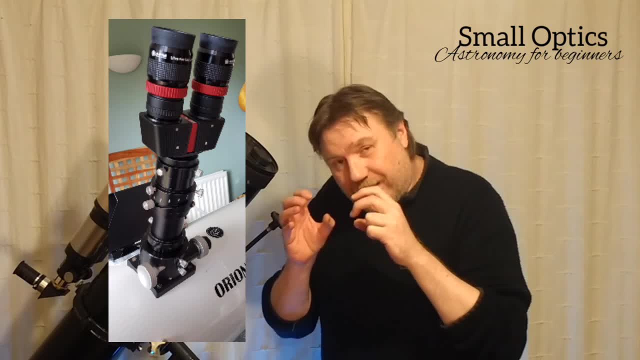 And you just put two of the same eyepiece in there And, uh, a lot of people say, oh, I can see so much better. We buy no viewers. It's not the case, Actually, they're seeing exactly the same. 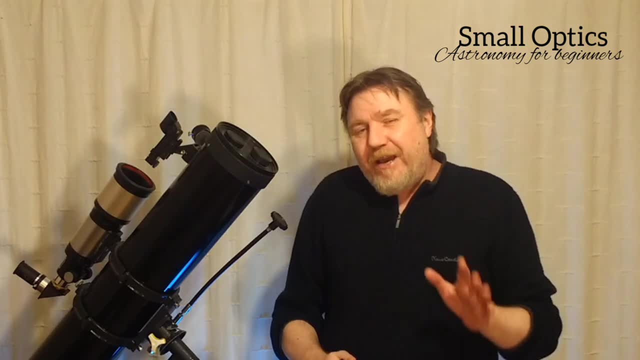 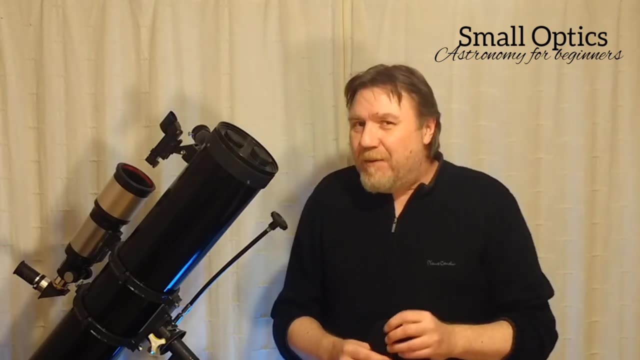 It's just that you've got both eyes open. Now it is a little bit of a technique to get used to this, And one thing that dramatically helps you are going to look like a bit of a pirate, but is to buy or make yourself an eye patch. 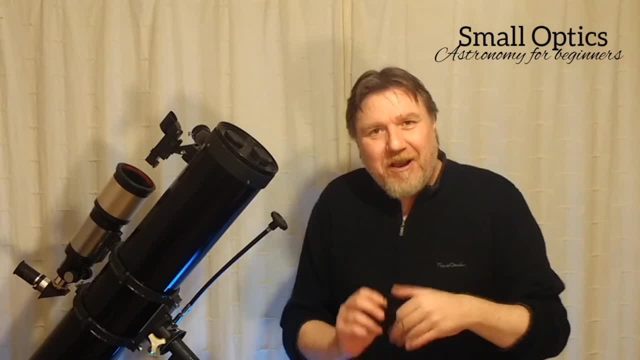 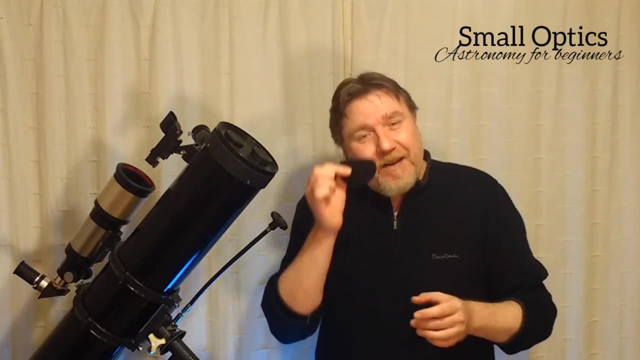 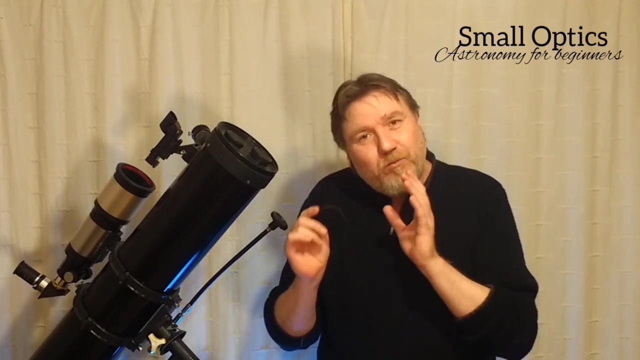 Okay, Uh, you may get a few People say, oh, what have you done to your eye? but, uh, you know you are in the dark, so but nobody's going to see you. Um, okay, And if you wear this over the over the eye that you don't obviously use for the eye, uh, uh, for the eyepiece, these, these really do help. 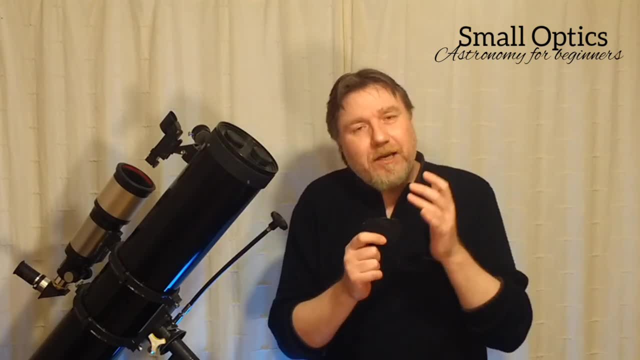 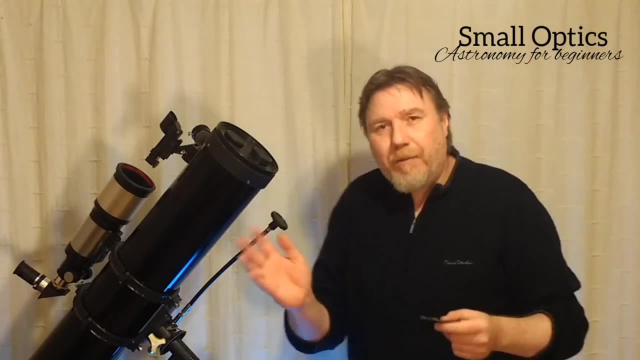 And, to be honest with you, I still use this. and where these uh come in handy is if you've got a lot of localized light pollution, And what I mean by that is street lamps nearby. You know there may be somebody's uh security light. 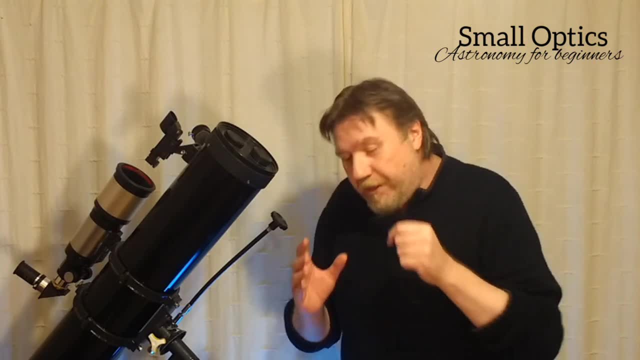 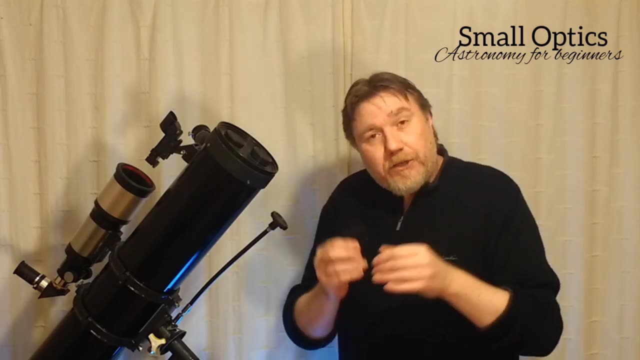 Yeah, That never turns off my problem. And, uh, when you've got both eyes open you have a you you've got a few distractions. you know you can see the reflections of this scope and things, Uh, so wearing an eye patch, uh, really does help this one. 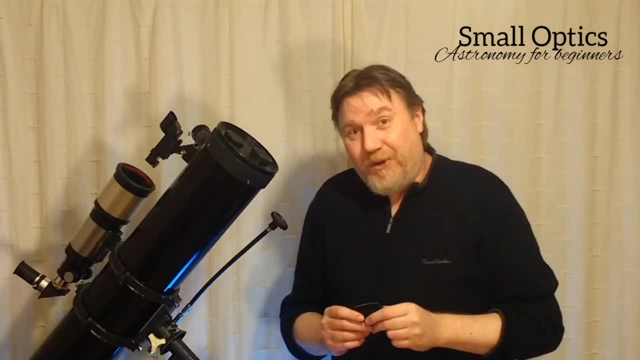 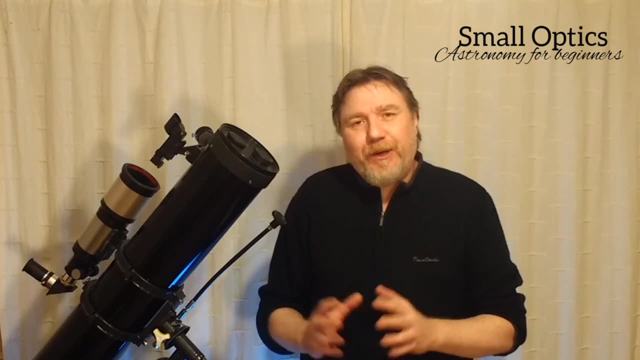 If there's one tip on this video that you need to try, you need to give this one a go. Okay, Number eight. Now here's another little technique that takes a little bit of getting used to, but, again, it's one of those techniques that, once you learn, you will always use. 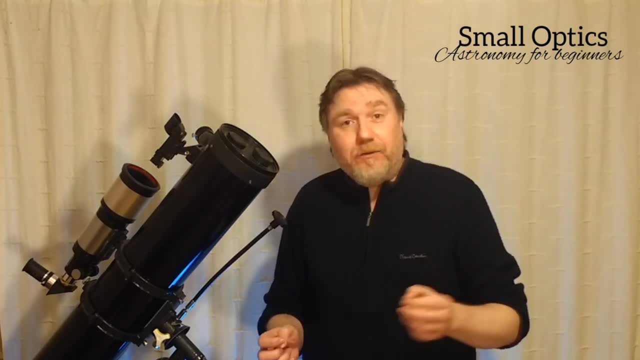 Now this, This one's especially useful if you like to look for some of the uh fainter objects, some of the Messier targets, uh, a few fainted galaxies and uh as such like, and that is to use what they call averted vision. 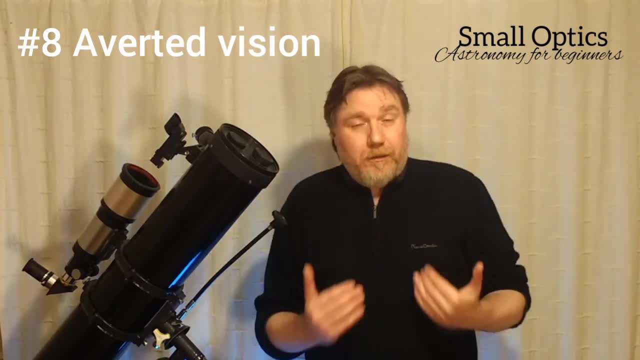 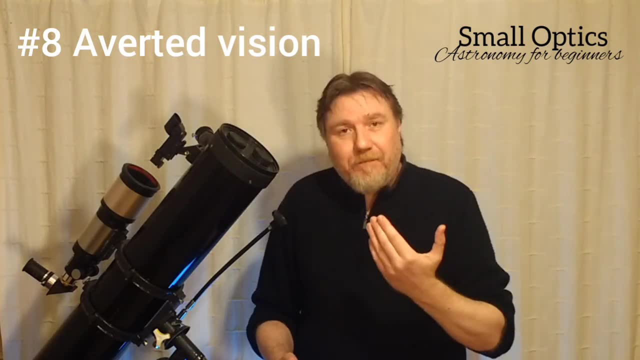 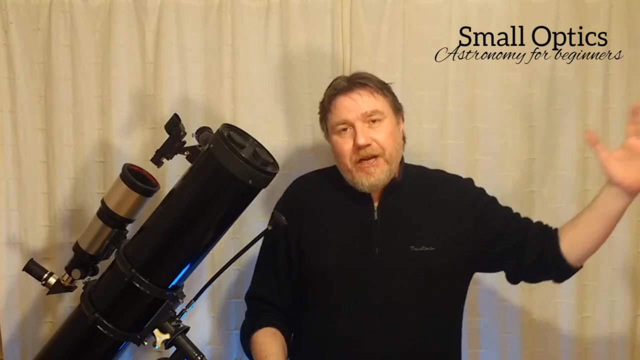 Okay. Now, this simply means is, if you look, you're looking straight at me, Okay, But be aware of everything else around you. Keep looking at me, Okay, And just be aware of everything around you, Okay. Another way you can test averted vision is by taking your hand out of view. 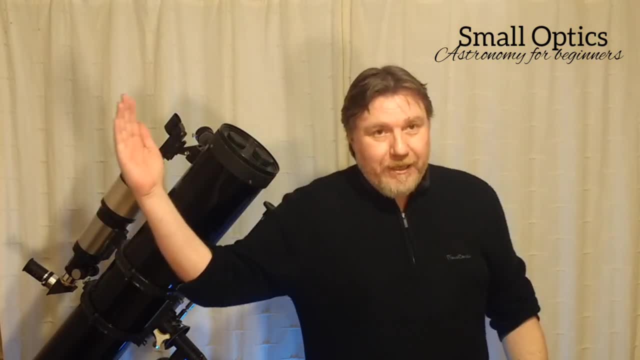 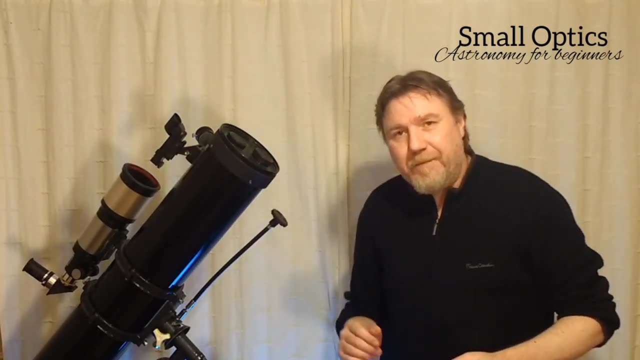 Yeah, And then not looking at your hand, but bring it in and keep concentrating on your hand. Okay, So you're like you're seeing it in the corner of your eye, if you like. Now, if you transfer this technique to the eyepiece, okay, 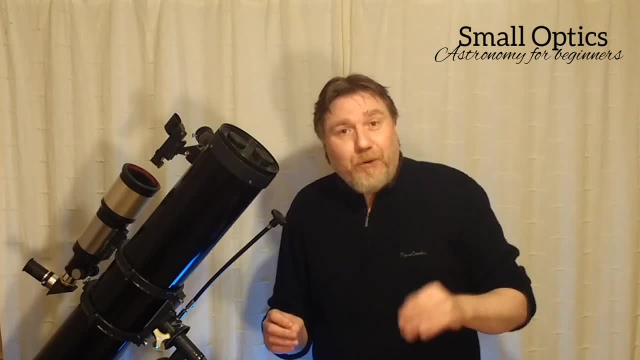 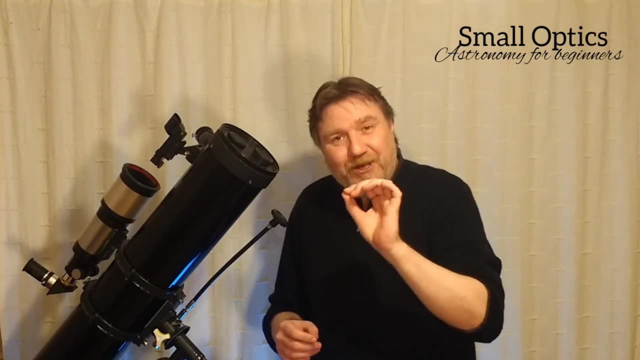 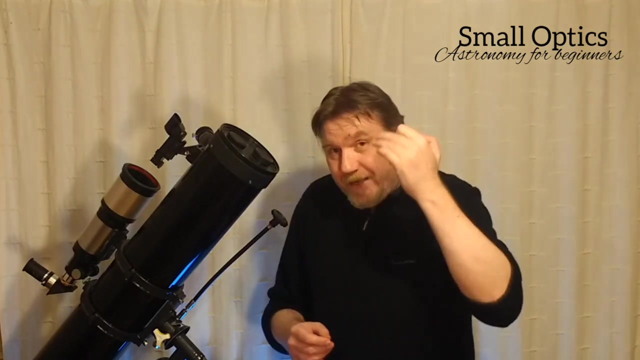 And this really works well for me. uh, on the ring nebula: Okay, Looking at the ring nebula, If you look at it direct, it's as though, Okay, It like comes in and out of vision. but using this averted technique, I'm just looking to just to the side of it and just getting it in a corner of the eye. if you like, you'll come really see the ring uh, pop out. 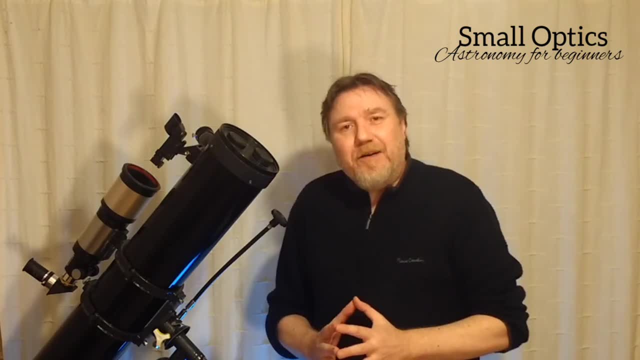 So again, a little technique for you to just try, um, and it's well worth your learning this one, learning the technique, and uh, just to make it a little easier, finding those faint fuzzies. Okay, Tip number nine. Now you really 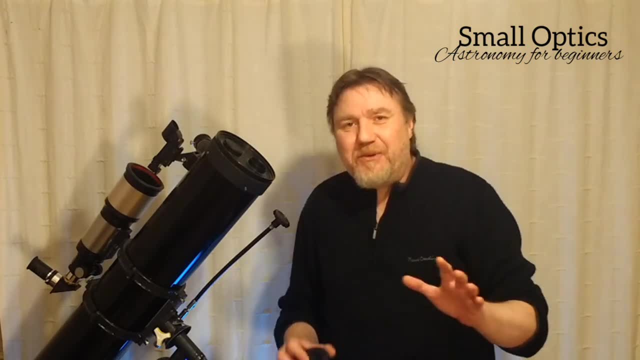 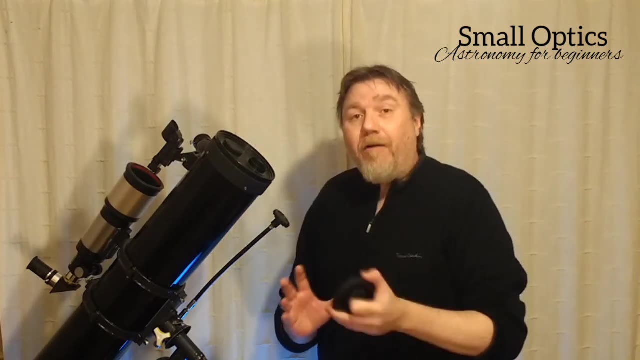 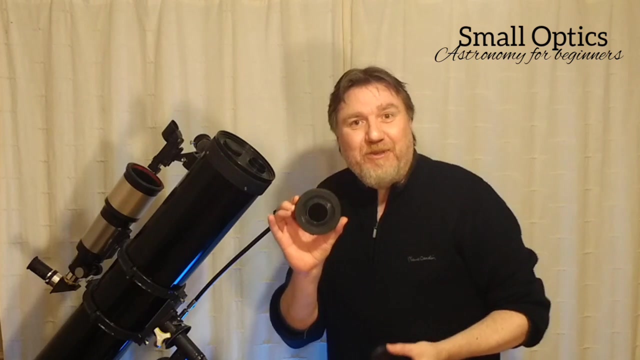 Are going to think I'm um trying to insult your intelligence on this one, And that is when it comes to dust covers and, trust me, people often ask about this center: um little, uh piece that comes off in the middle. 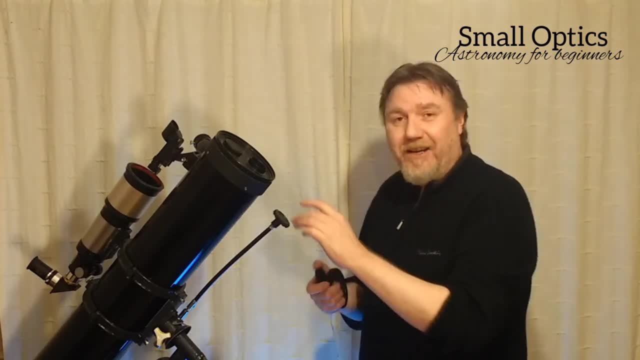 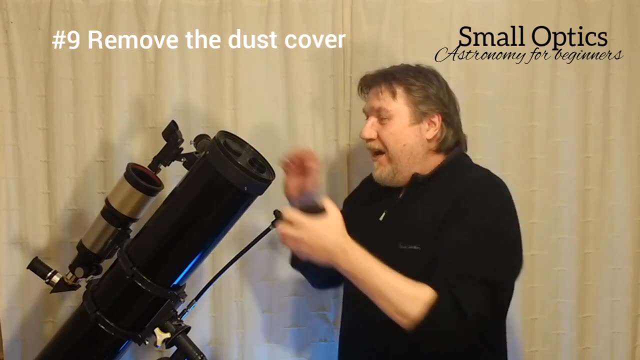 And it's quite a mystery to to uh people who are new to the uh hobby. but, um, you need to remove all the discover. Okay, Um, that includes you know You take the whole thing off. 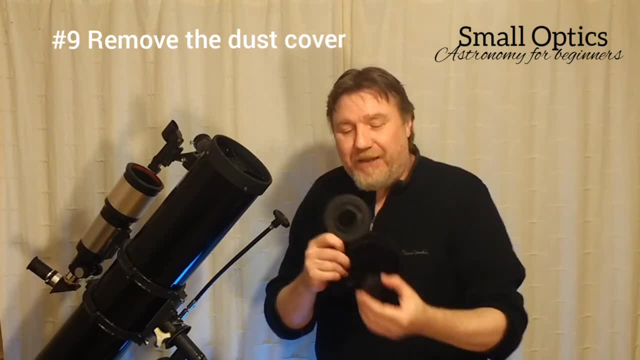 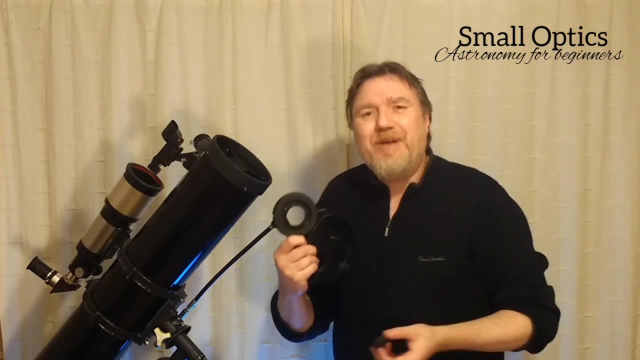 It's not just this uh little little little center bit in the middle. Okay, That uh people have. I've asked me over the years, you know, do you know that that, that little bit? do I leave that on or do I leave it off? 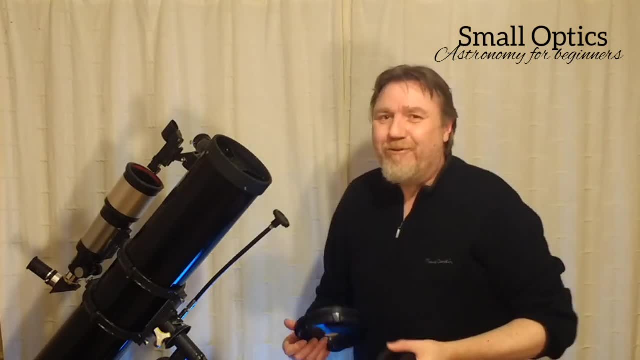 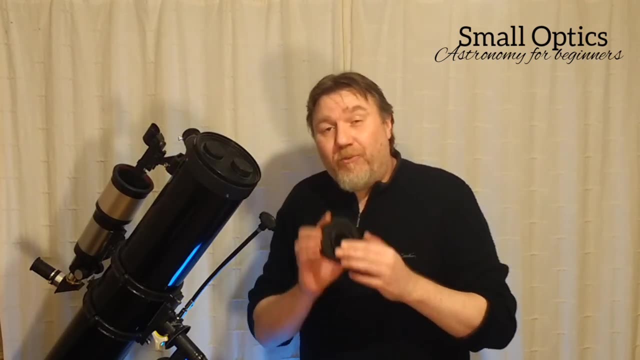 So remember to take the entire cover off. Okay, Now tip number 10, we'll let it stay on. dust covers And uh, you may have been asking yourself, well, why do they leave this? uh, you know, this whole, this separate thing that has a cap on it. 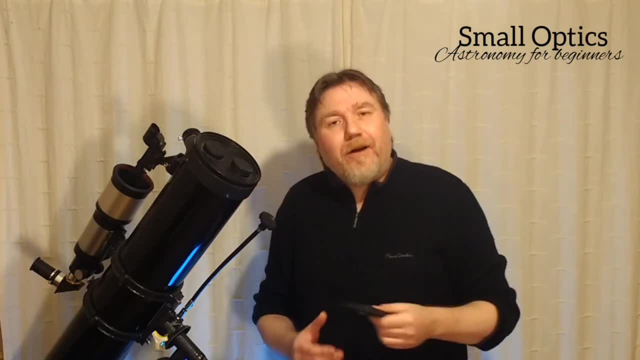 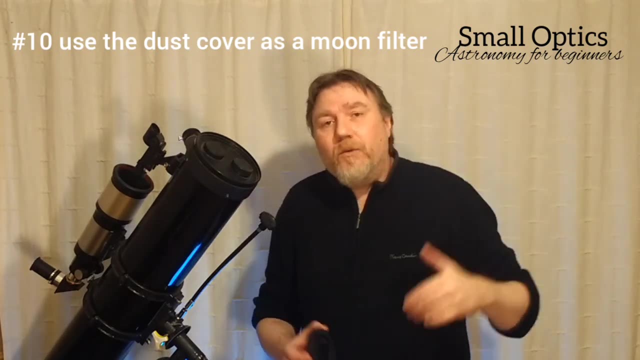 Well, this is, This is like an aperture stop, And if you haven't got a uh moon filter, say if you actually do leave this on, because the moon is a big bright object. we don't need much light from the moon, because it's it's generating it off. 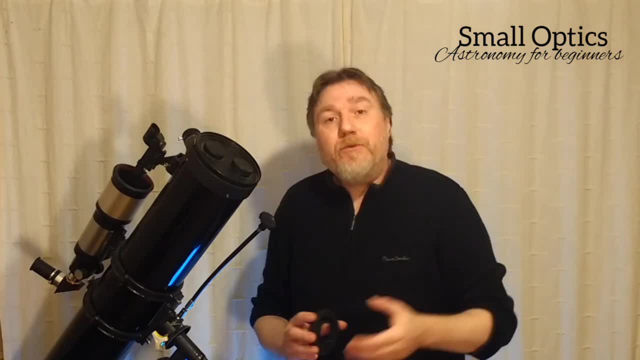 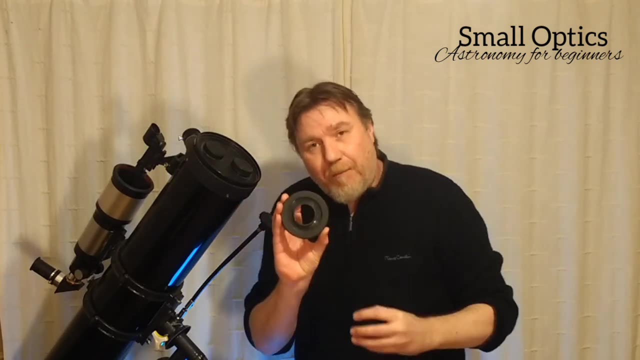 And it can be really dazzling at times- the moon, especially if you don't use a uh a filter. And if you haven't got a filter, leave it on. in this way, you take your center cap off and leave it on.